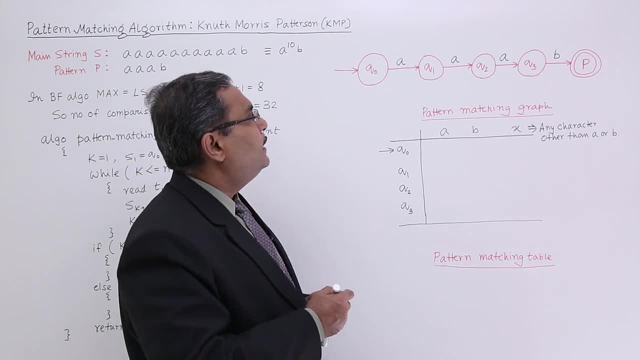 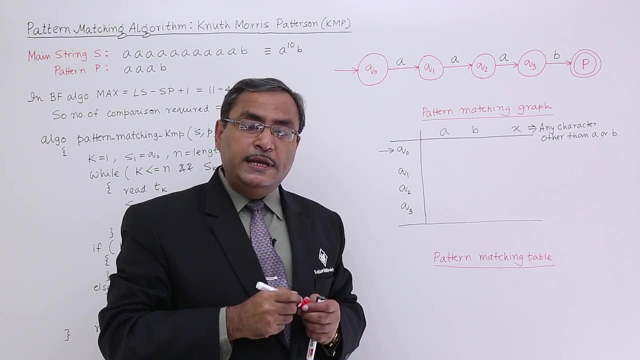 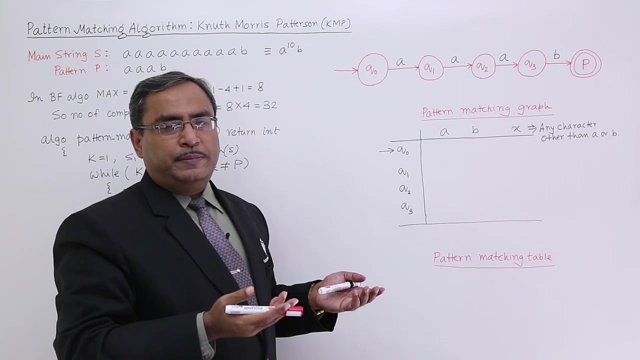 transition system. So now let me see that if I get A, then I shall move to Q1?. But if I get A, if I get B in the main string as the beginning character to do the comprising pattern, then then I should stay with Q0.. That means I should stay with it because I should. 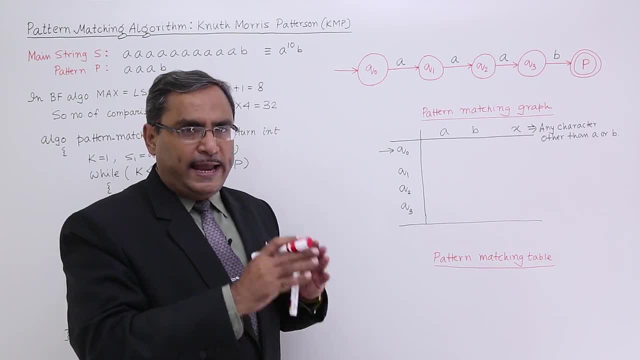 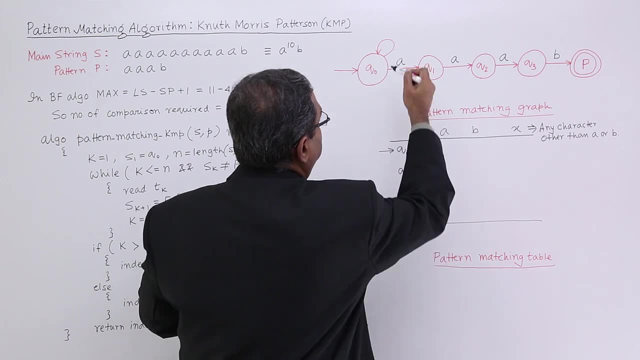 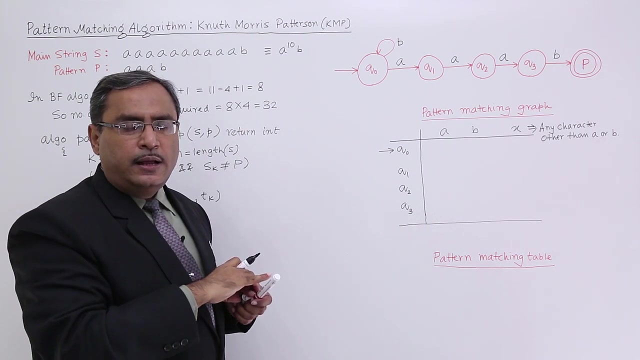 wait for A, because my pattern starts at A only, So I am writing this one in this way. So for this one I shall have this: A B, B, like A, B, because A, A, only A, B B pattern is having the character b. that means if the main string is having the character b. 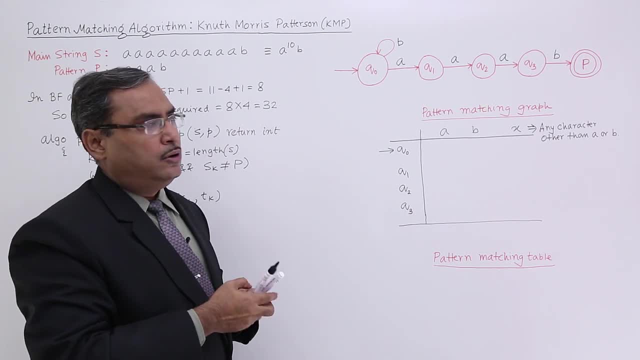 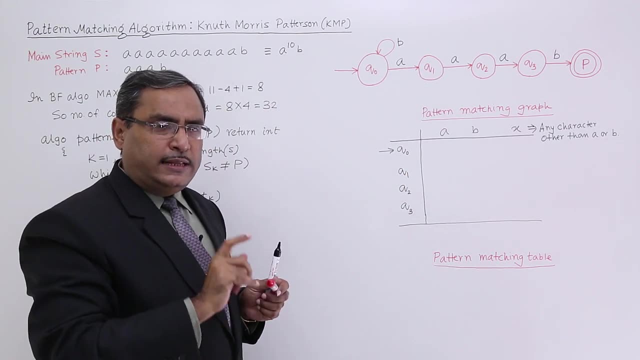 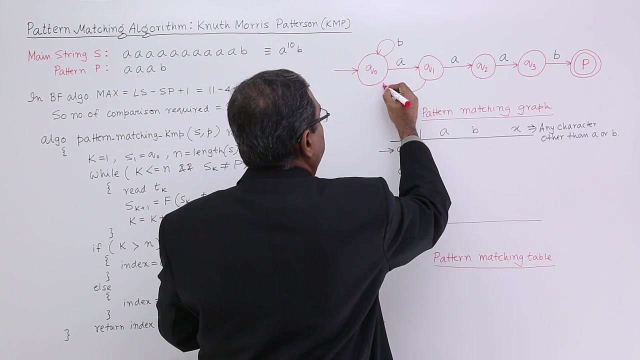 that means the pattern has got not initiated yet. okay now q1 means i have recognized a. now if i recognize b now in the main string, that means i have recognized a. b means no issues. so that means i should get back to q0 if i get b. 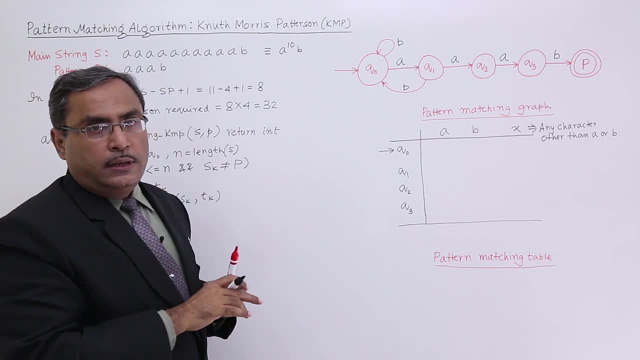 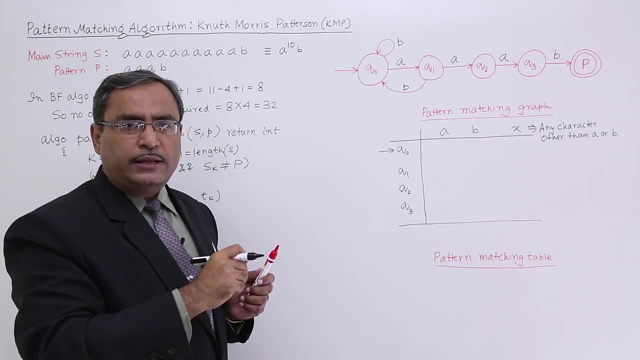 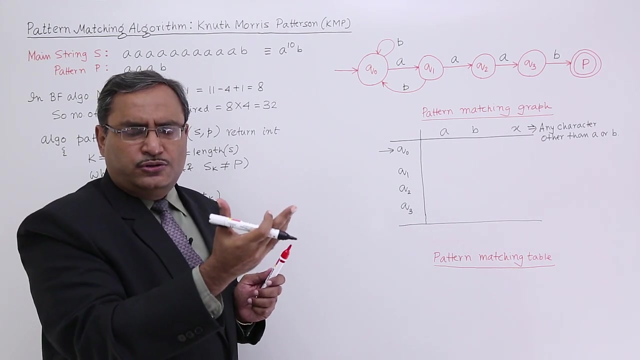 when at the state q2 i have recognized a- a. now if i recognize b in the main string, that means in total i have recognized a, a, b and that is not the substring of the pattern also. so that means i should retrace back to q0. that means the pattern has got got. has got not. 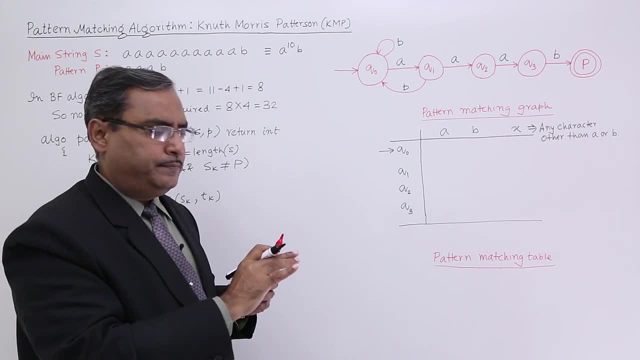 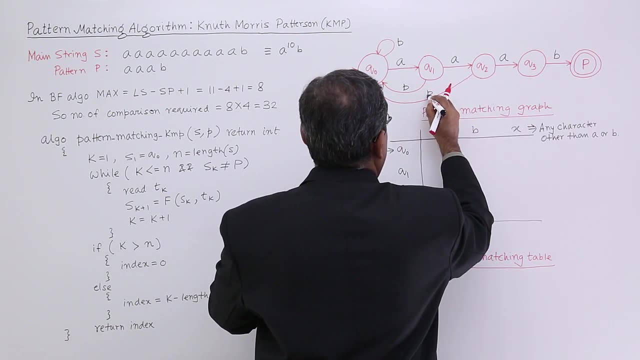 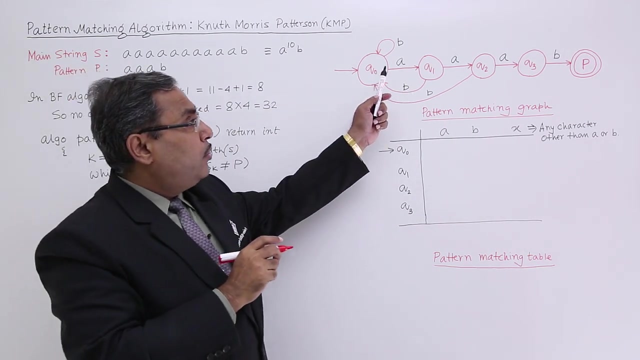 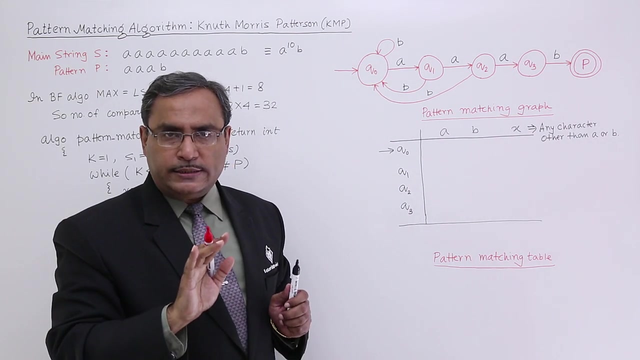 recognized and not even the substring of the pattern. so i should go back to q0 when i am reaching at q3. when i am reaching at q3, that means i have recognized a, a, a. if i get b then i shall recognize that it is my pattern i have recognized. but if i recognize a, 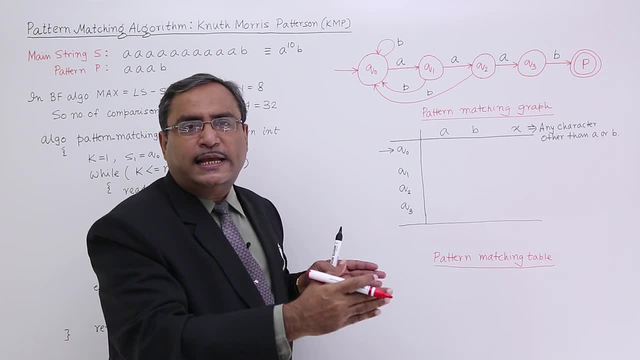 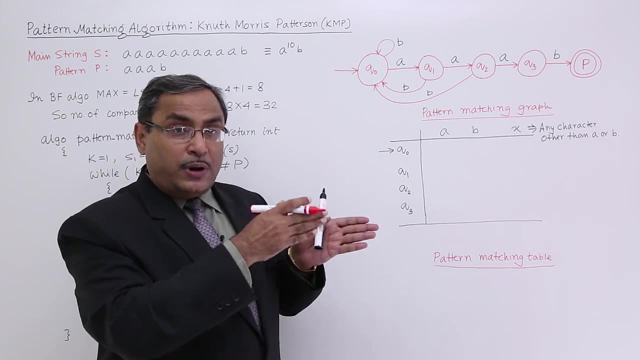 that means what that means. i have recognized four times a, three times here and one times a here. so four times a means discard the first time A. So I have already recognized 3 times A. So I require only one B to reach to P. So 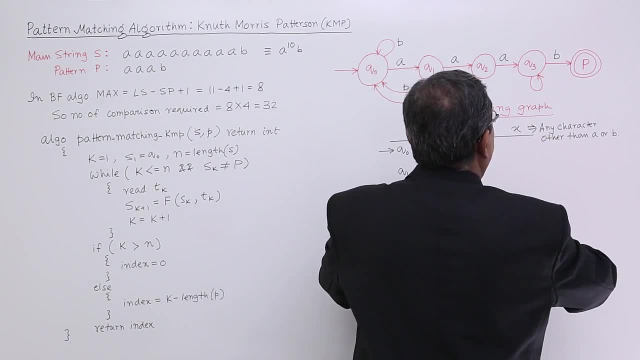 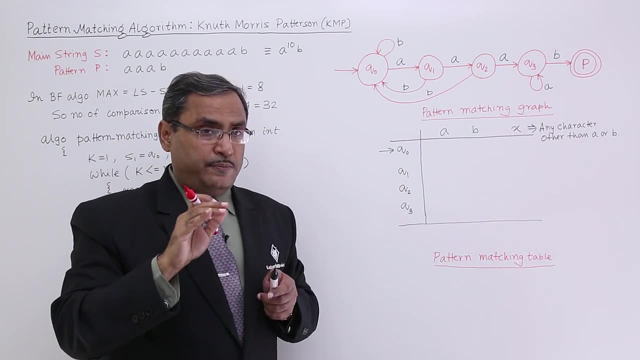 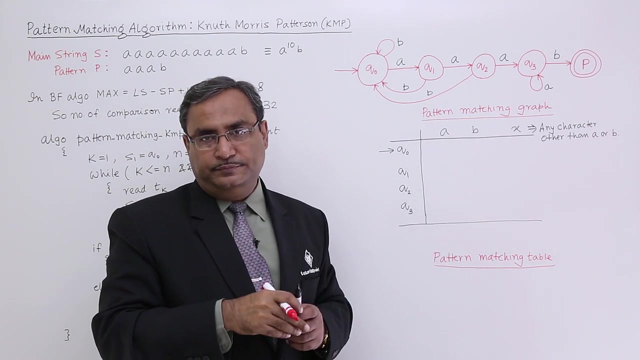 that means I should stay back here with the input A. So I think you are getting this logic. Please do such practice with other patterns also. Say pattern like A, B, A, B. Try to draw the respective pattern matching graph. So again I am repeating From Q 0 to Q 1. 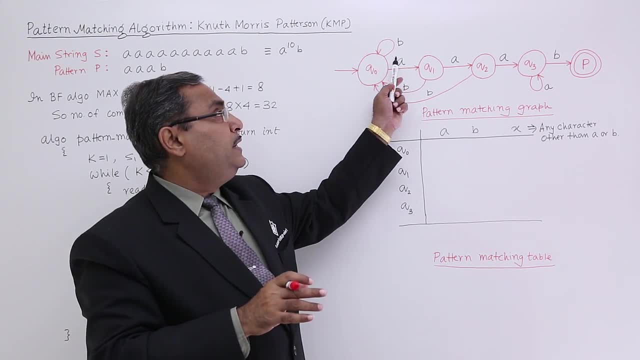 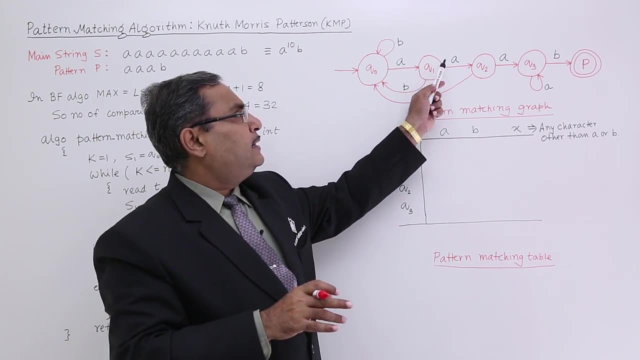 I require one A in the main string. But if I get B, I should stay, remain with Q 0.. When I am at this Q 1, that means I have recognized A. So if I recognize another time A, So I should move to next state, Q 2.. But if I get B, that means I have got A B, that is not. 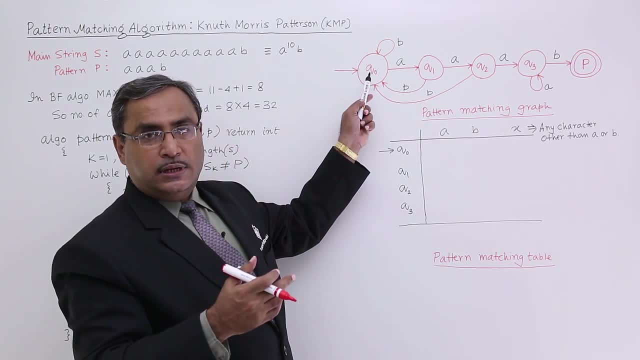 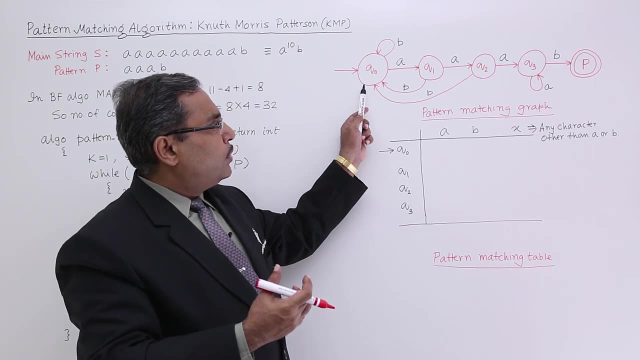 a substring of the main pattern, So I should go back to this. Substring means not beginning substring of the main pattern, So I should go back to Q 0.. In this way, up to this, it is okay. But here, after getting B, I shall go to the. 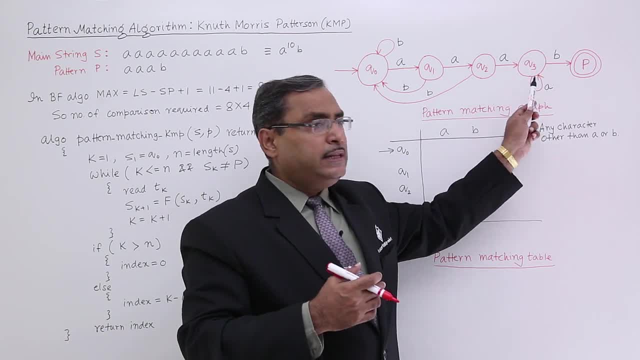 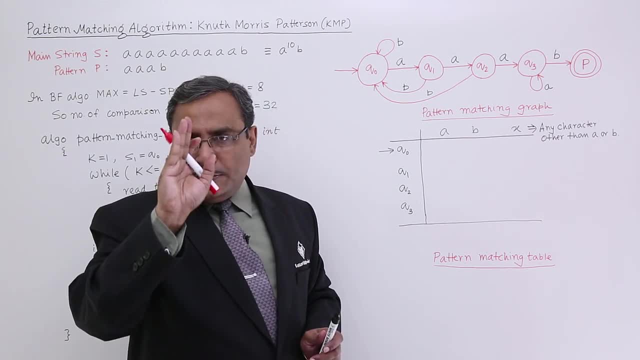 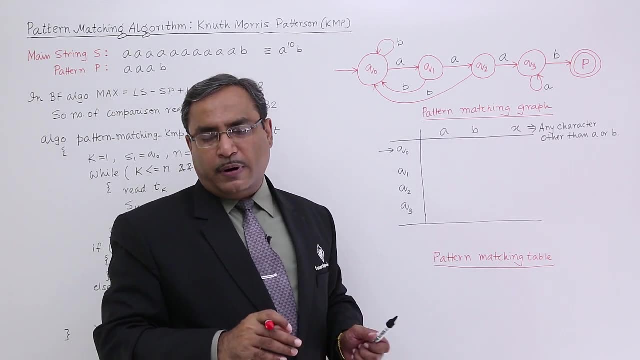 already I have got at least 3 A's, Sorry. I am just waiting for B to recognize the pattern. So this is my transition. a system or pattern matching graph, but you cannot feed this particular graph to your algorithm, So that is why let me convert it to the respective pattern matching. 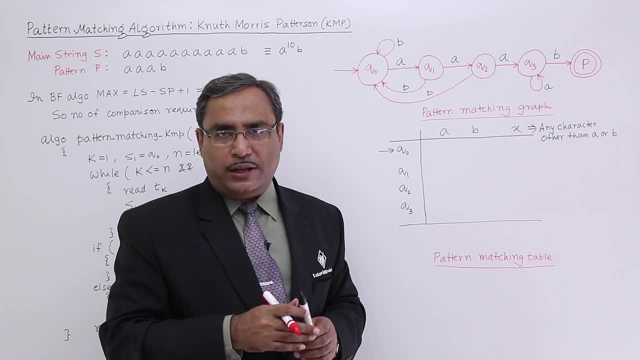 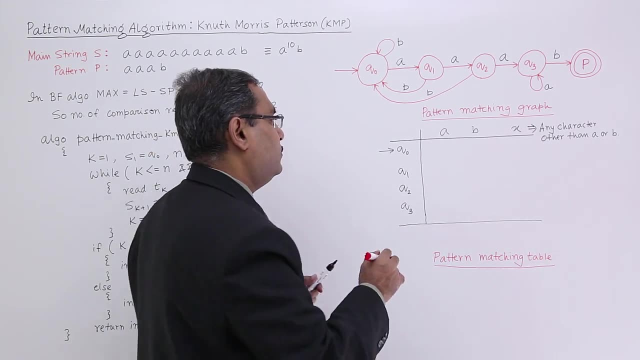 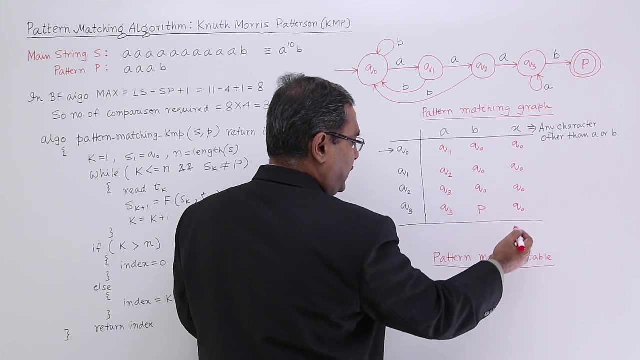 table or transition table. okay, Now see what I am writing. See here. So see, here is the goal. So this is my result: null. So I am saying that this two E G now is equal to 8. So now, in this way, this pattern matching table has been constructed. Actually, I have. 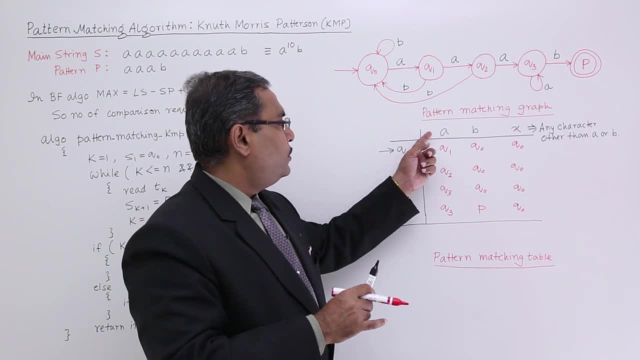 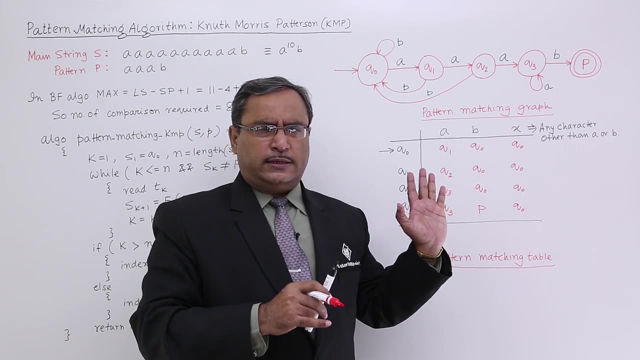 done the same thing. So q0, a, q1, q0, a, q1, q0, b, q0, q0, b, q0.. x means any other character other than a and b, any character other than a and b. Obviously, I shall be. 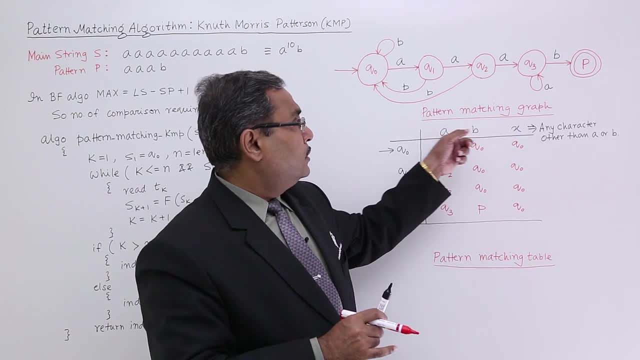 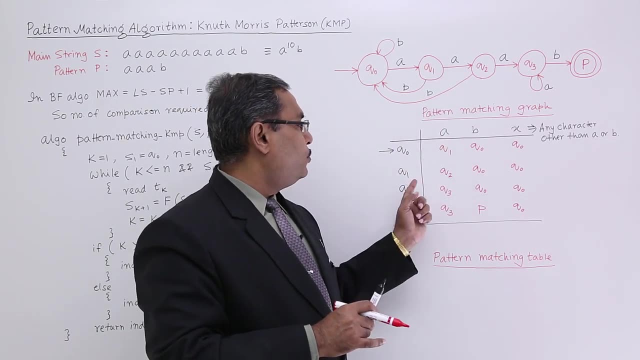 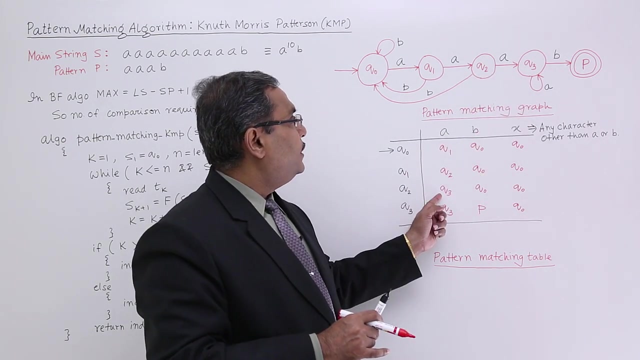 returning back to q0.. So that is no issues, because I should return back to q0.. And then q1, a q2, q1, a q2, q1, b q0, q1, b q0. So this: q0, q2, q2, a q3, q2, a q3.. So 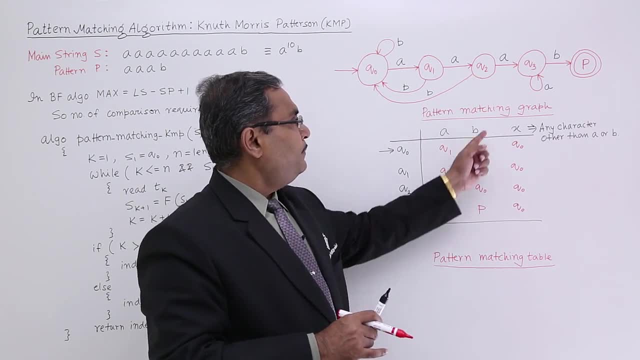 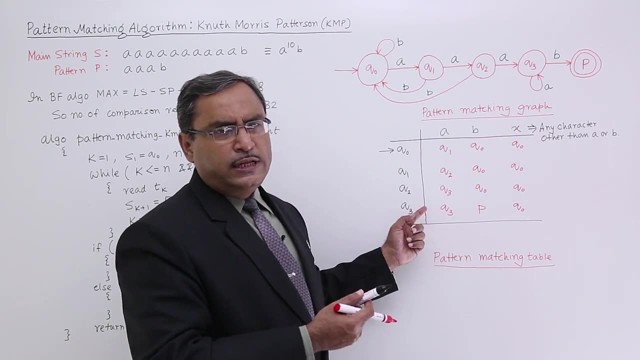 q2, b, q0,, q2, b, q0.. Last one, you see q3, b pattern, q3, b pattern and q3, a, q3, q3, a, q3.. So in this way I have written the same. So now this is a table which we can. 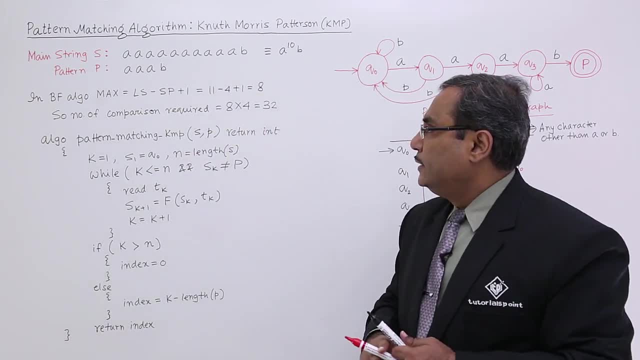 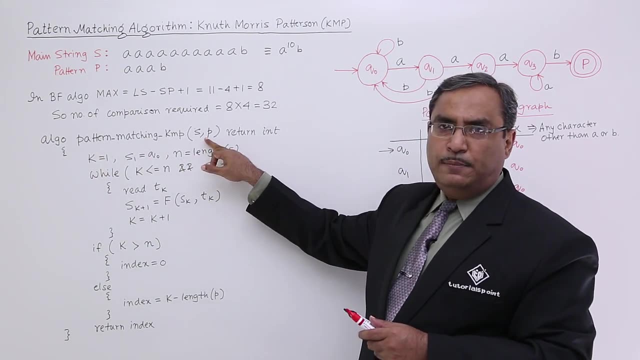 feed to my algorithm. Now let me come. Let me come to the algorithm. So algorithm pattern matching k and p. I am passing this s and p. Here I am having two p's. One p is this one, One p is this one, Another p. 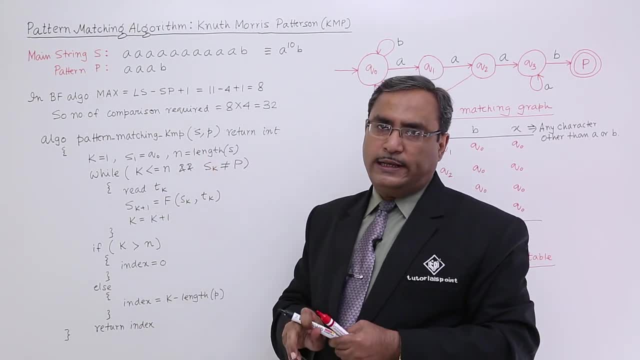 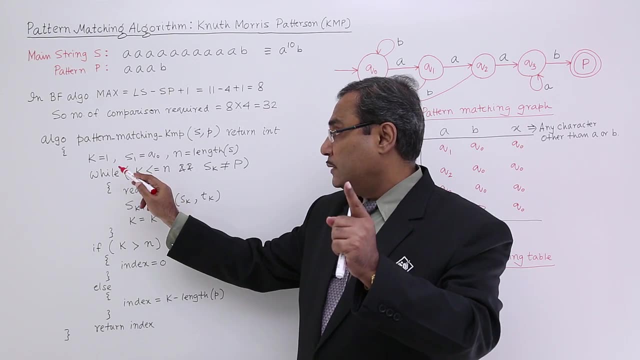 is this one. Remember this pattern. I am writing this one in lowercase letters. Okay, Now see, k is equal to 1.. That means at the first position of the string I am going for the path checking. s1 is equal to q0. So initial state sk. you can also write s1. So initial. 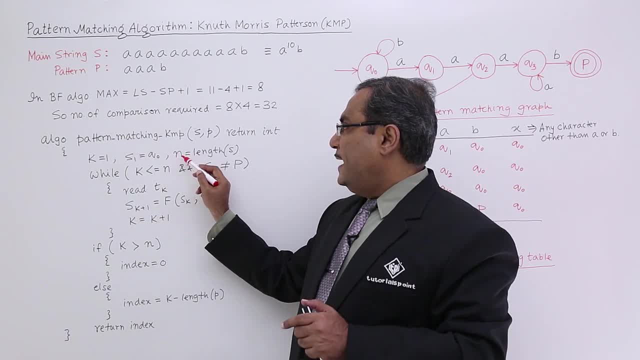 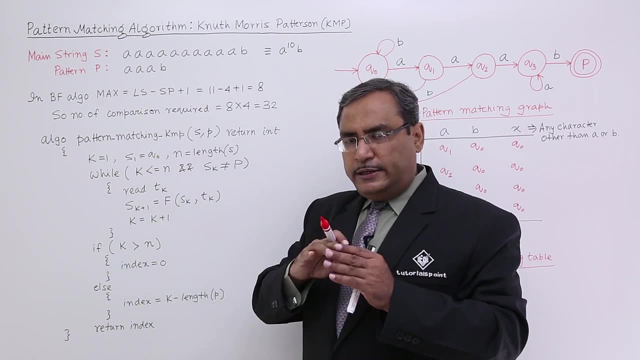 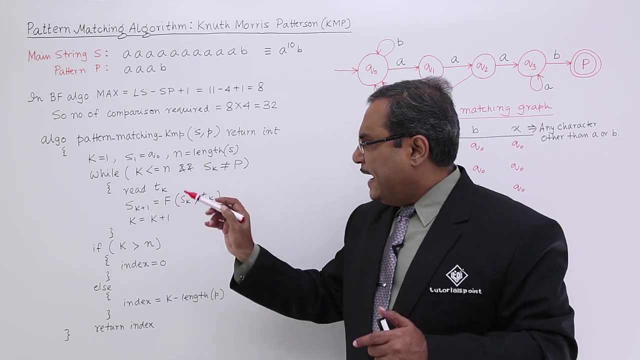 state sk, because k is equal to 1, here is equal to q0.. n is equal to length of the string. Okay, While k is less than equal to n, that means until I exhaust or search the full string. So, while k is less than equal to n, I can continue. And this kth state is not a pattern. 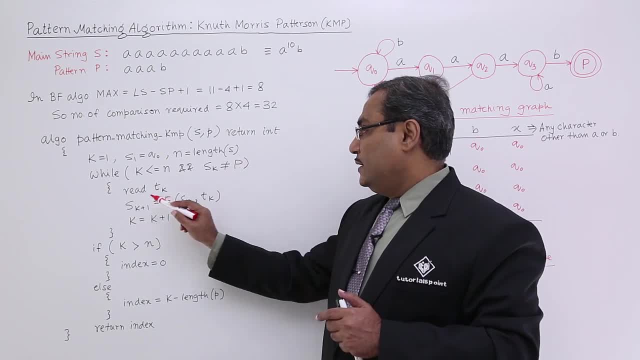 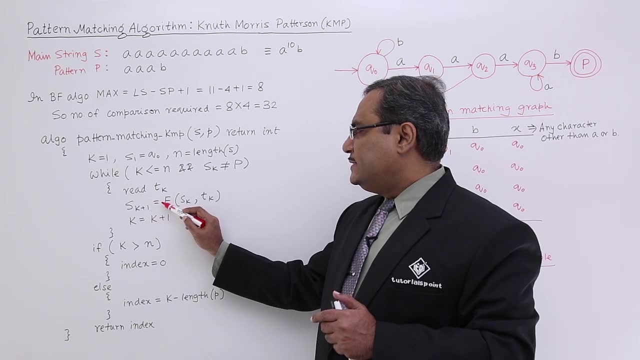 Until the kth state is not a pattern, read tk. So read the character from the kth place of the pattern. So read the character from the kth place of the pattern. So read the main string. sk plus 1 is equal to f. What is f? This particular pattern matching table. 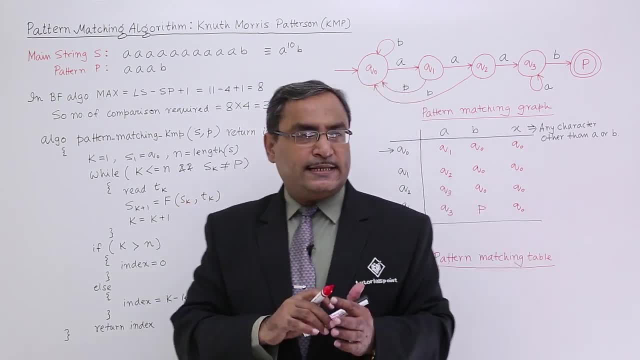 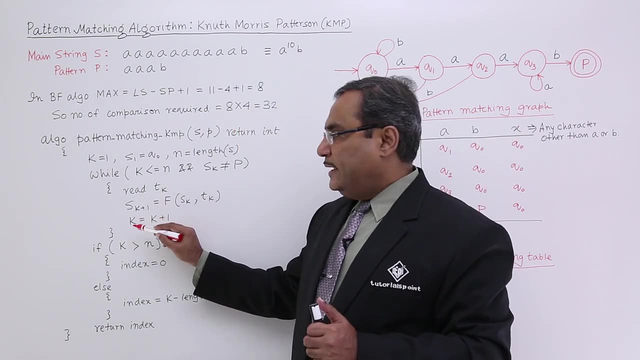 is my f, So f, sk, tk. What is sk? That is the state. What is tk? That is the character red. So that will give me the next state: k is equal to k plus 1.. So in this way I 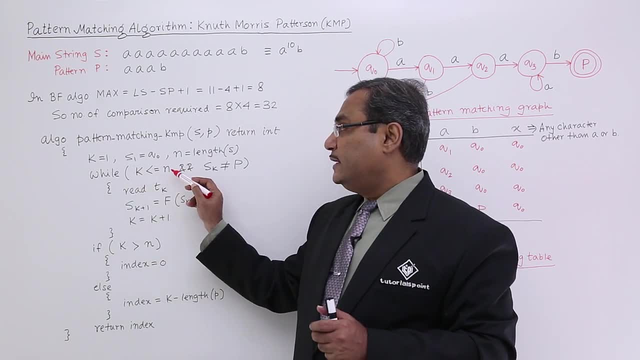 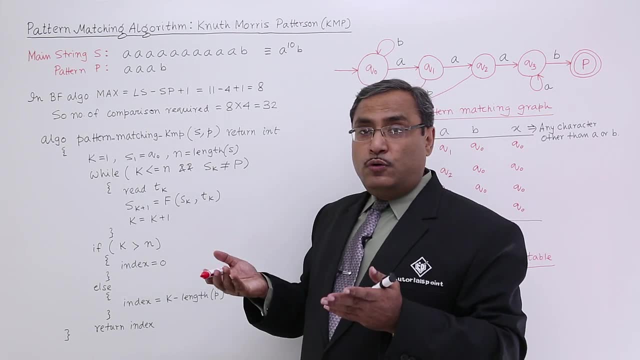 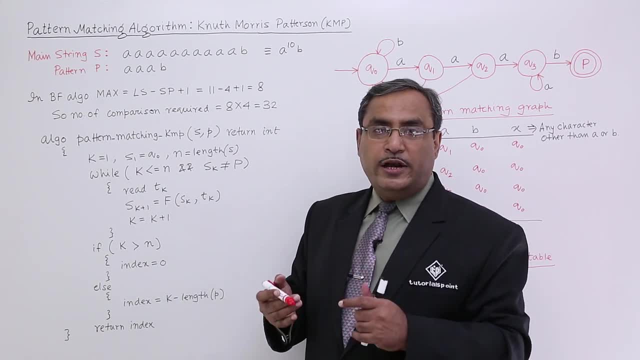 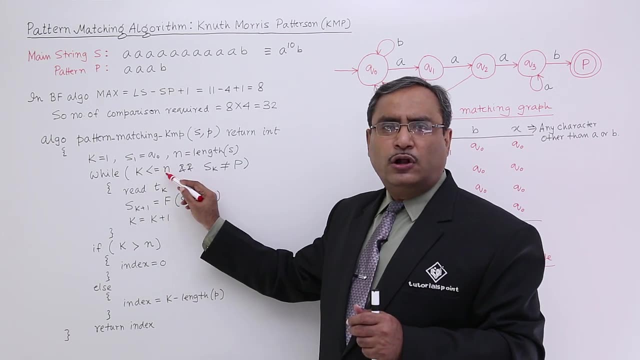 not know. So I do not know, So, I do not know. So for which reason this, while block has got terminated. So after coming out, I am checking- Is k greater than n. That means it has come out only due to this false. So that means index is equal to 0.. The pattern: